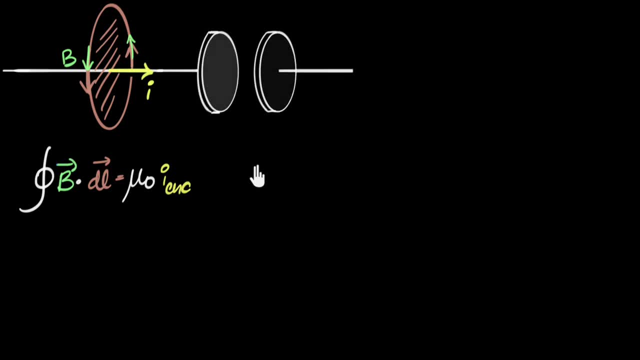 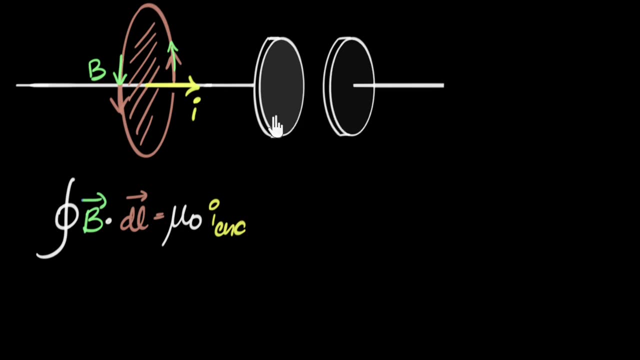 with a charging or discharging capacitor, And let's zoom in a little bit so we can see better. All right, So we have imagine two circular plates of a capacitor, and let's say that our current over here is increasing, Just for the sake of example. 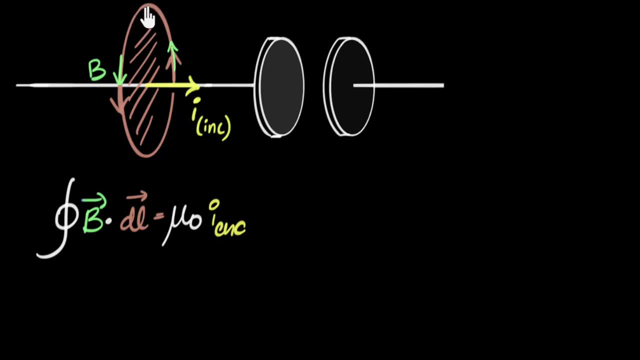 So the capacitor is charging, And now what we'll do is we'll focus on two points: One point over here, let's call that point P, and another point somewhere in between the capacitor, but at the same height, Let's call that point Q. 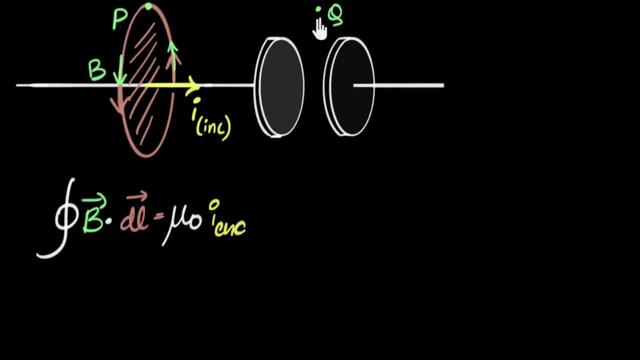 I want us to think about what is the magnetic field at point P and point Q? according to Ampere's Law? We don't have to calculate it, but let's just compare them. So if I were to calculate the magnetic field at point P, 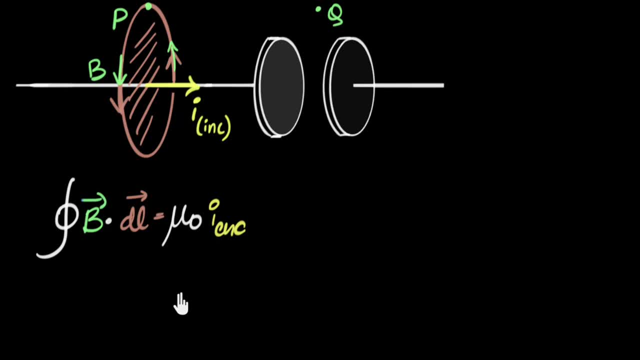 using Ampere's Law. I would have to calculate the magnetic field at point P using Ampere's Law. I would get some answer, some non-zero answer. That's important, right, Because it's enclosing some current. What would I get if I were to use Ampere's Law here? 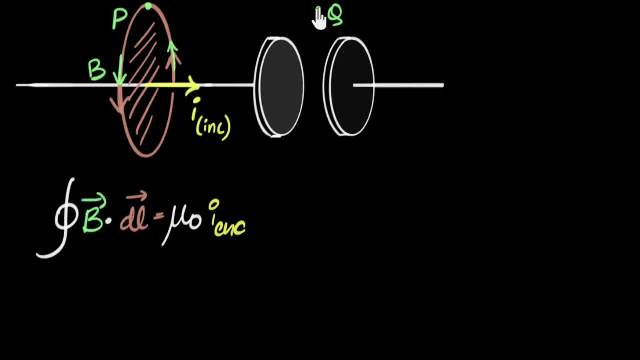 Well, let's see. I'll again choose a circular loop, because everything is nice and symmetric. So if I go ahead and draw a circle, a closed circular loop, attach a flat surface, And if I apply Ampere's Law over here, 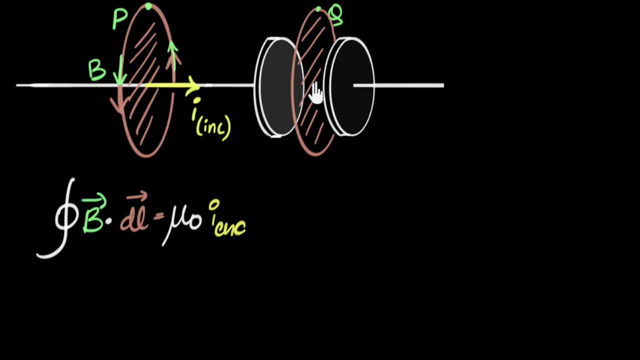 the one thing that I see is that there is no current passing through this surface. Why not? Because this loop is right in between the two plates of a capacitor and there is no current over here. It's vacuum, Which means, if I apply Ampere's Law, 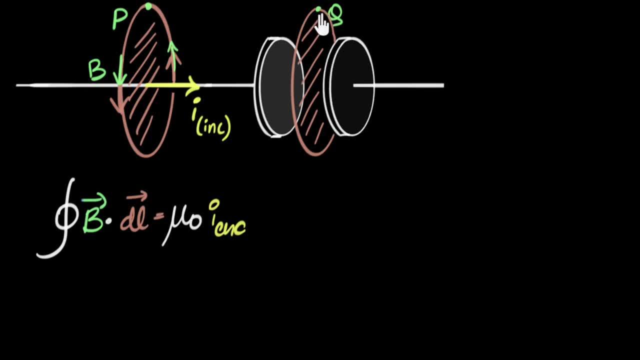 the right-hand side becomes zero, which means Ampere is saying the magnetic field over here is zero. Magnetic field according to Ampere's Law at point Q is zero. And that's the problem, because experiment says that's wrong. According to the experiment. 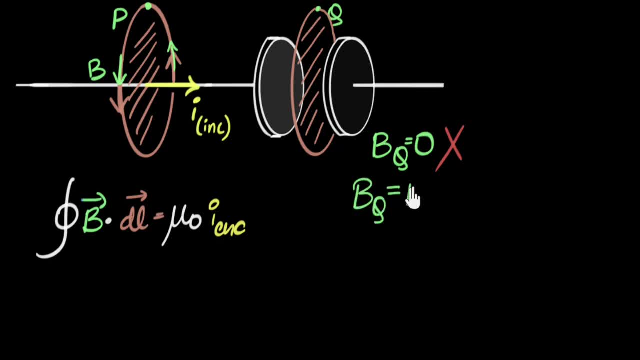 magnetic field at point Q is pretty much the same as magnetic field at point P. That's what experiments tell us And that is the problem with Ampere's Law. So you can see there is some problem with Ampere's Law because it's not giving us the right answer. 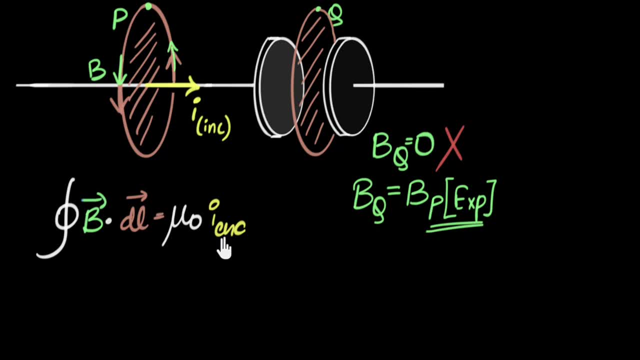 in this situation. So there is some fundamental problem with it. But what is it For that? let's go one step deeper, beyond mathematics, and see what this equation is telling us. You see, if you asked Ampere, let's go and ask Ampere. hey, Ampere, if you ask Ampere. 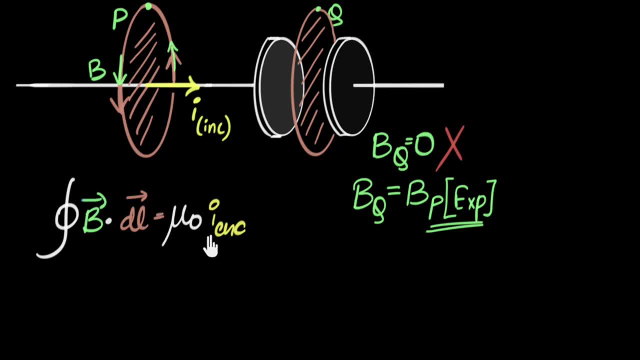 if you ask him what generates magnetic field, Ampere says currents. And that's why in his equation he's saying: look, your loop should enclose some current. only then there will be magnetic fields. If you don't enclose, you will not get magnetic field. 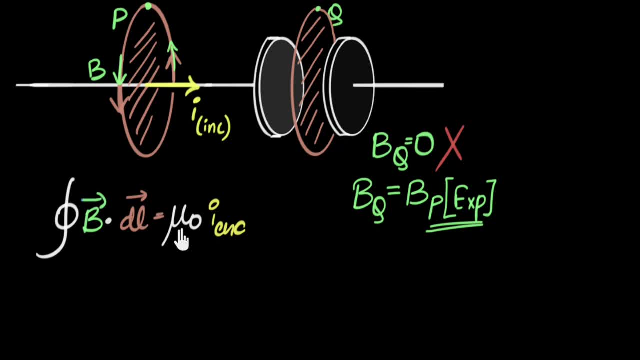 And it's for that reason. Ampere or, for that matter, any other scientist back then would say that you get zero magnetic field. they're predicting zero magnetic field over here because it's not enclosing a current, Because no current, no magnetic field. 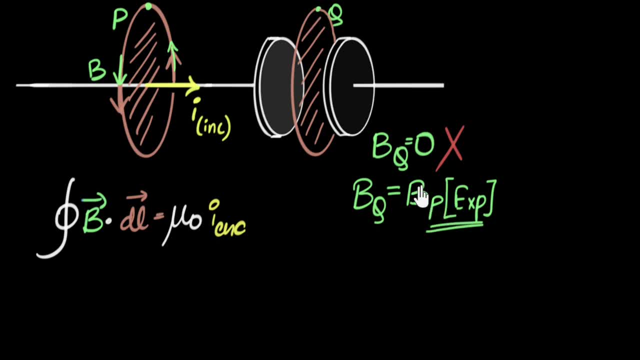 But we do know that there is no magnetic field. But we do get a magnetic field experimentally. So the question is: why is that happening? This is where Maxwell steps in. Maxwell says: maybe current is not the only thing that generates magnetic field. 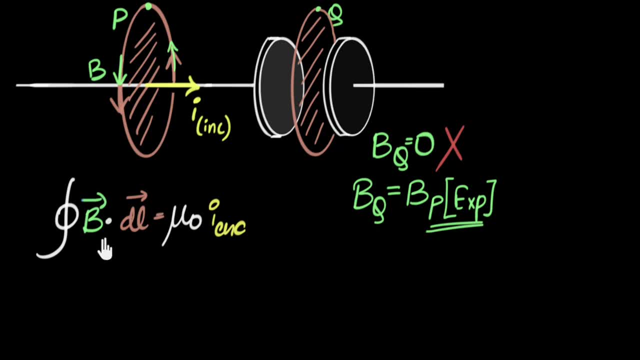 Maybe there's something else that's generating magnetic fields which is missing in this equation. And I'm sure at this point you would get up and you would ask Maxwell what else can generate magnetic field besides current? And Maxwell says I won't tell you the answer right away. 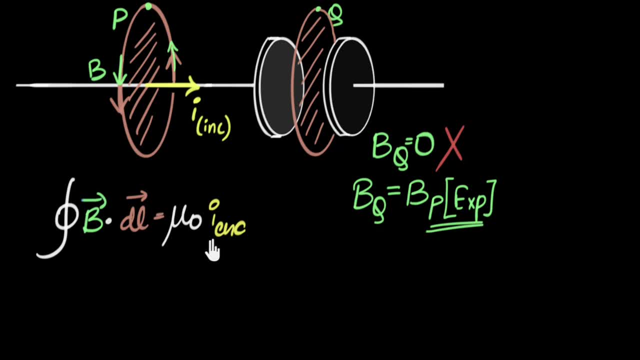 I actually want to walk you through the thought process that maybe Maxwell had to give you an opportunity to guess what that other way could be. So let me zoom out. and let me just walk you through the process. So Maxwell is saying: let's zoom out. 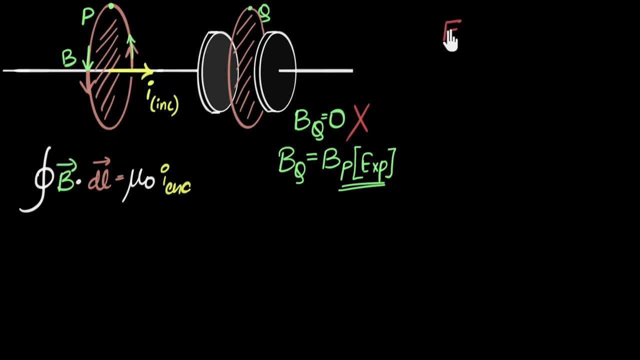 Let's recap a little bit. If we go back to electric fields- electric fields- and we ask ourselves what generates electric fields, What creates electric fields, What's the answer for that? Well, we have studied: electric fields come from charges. 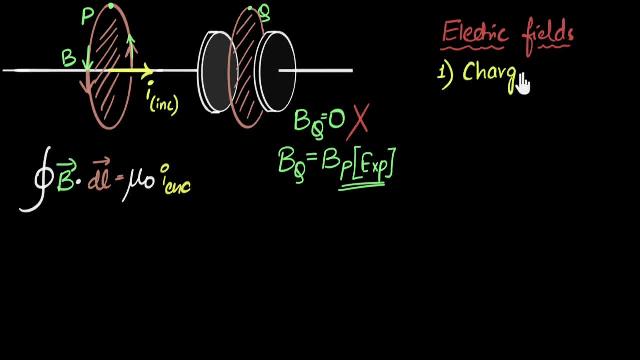 positive and negative charges. right, Charges generate electric fields, But we saw there's another way to generate electric field even without charges. Remember, Faraday showed us that. Faraday showed us that you can generate electric field by changing magnetic flux. 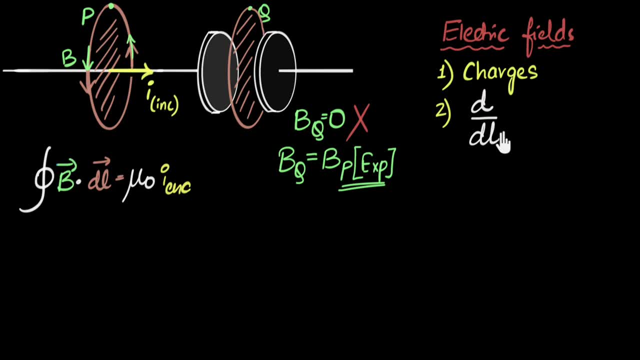 So let me write that You can also generate electric fields by changing magnetic flux, And we call this electromagnetic induction. We talked about all the cool applications of that, So there are two ways of generating electric fields. Now, similarly, we come to magnetic fields. magnetic fields. 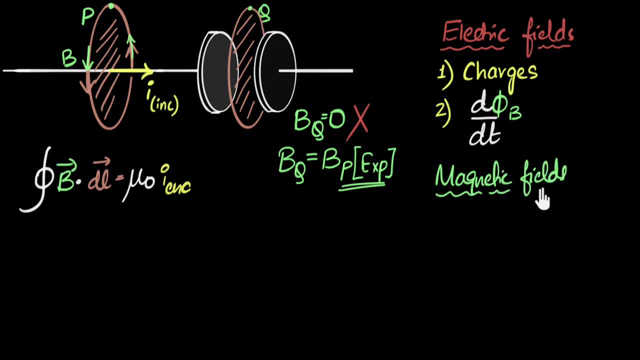 And we ask ourselves: hey, what generates magnetic fields? What's the source for that? And so far we had only one answer for that: Current Current. Currents generate magnetic field. Currents are moving charges And that's why the unit name was called. 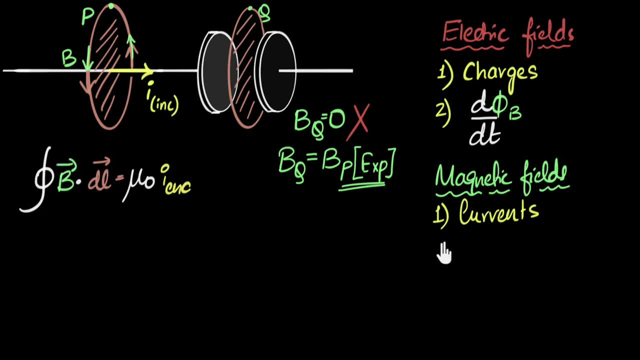 moving charges and magnetism. But now Maxwell is coming in and thinking: maybe there's another way to generate magnetic field which is similar to this. Now can you pause and think about what that other way could be? I want you to guess this. 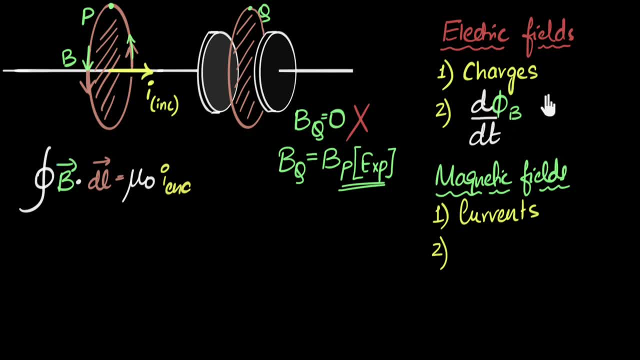 All right. So changing magnetic flux can produce, can produce electric fields. So Maxwell is thinking: maybe changing electric flux, changing electric flux, can produce magnetic fields, Maybe that's another way of generating magnetic fields. Ooh, How does that answer this question? 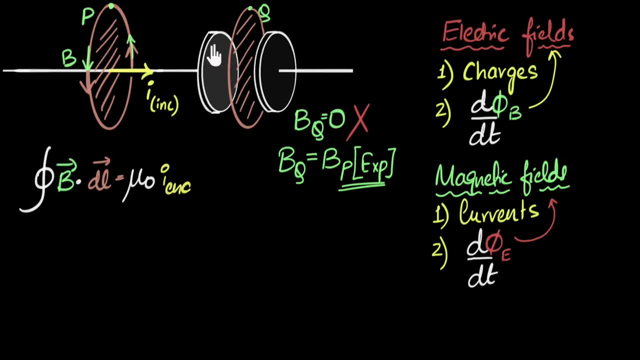 Well, you can see, as the capacitor is getting charged, there is an electric field that's being generated over here And as the charge is increasing, that electric field is increasing And because the electric field is increasing, the flux through this loop is increasing. 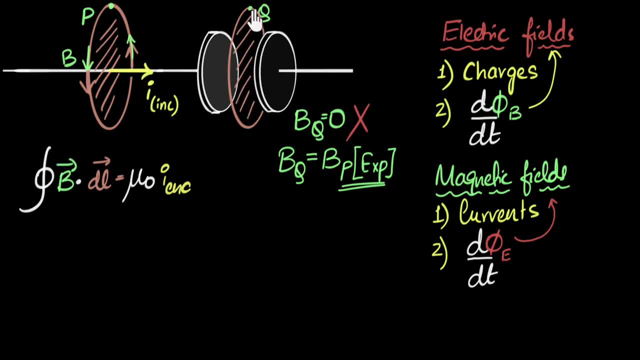 And Maxwell is arguing and saying: because the flux is increasing, that's why there's a magnetic field generated over here which is missing. over here, the term is missing. And so what Maxwell does is he adds that other term. He says: 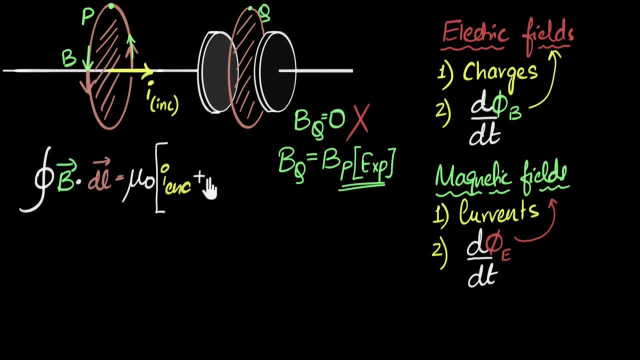 there needs to be another term which takes care of the changing electric flux, And we're not going to go through the derivation. the other term happens to be epsilon, naught times d over dt of electric flux, And this now is what Maxwell says is the complete equation. So this equation takes care of both the 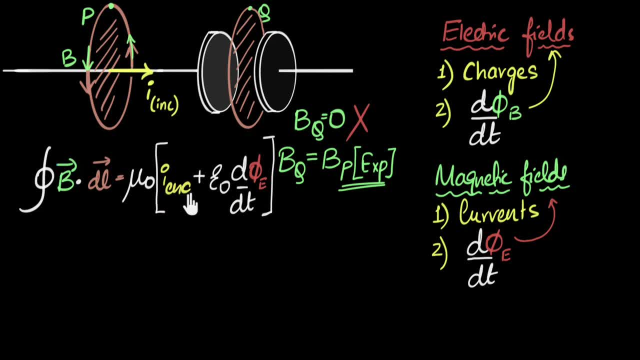 sources. You get magnetic fields due to currents and you get magnetic fields due to changing electric fluxes. This complete equation is now called Ampere Maxwell's law, for obvious reason, because Maxwell completed it. And finally, what do you think is the unit of this term that Maxwell? 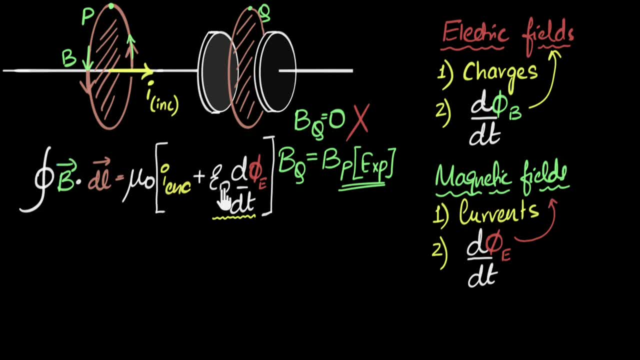 added. Well, at first I would think that, oh my God, so much calculations. unit of epsilon naught multiplied by units of phi. But another way to think about it is: remember you can only add two physical quantities which have the same units, which means this should have the same units as: 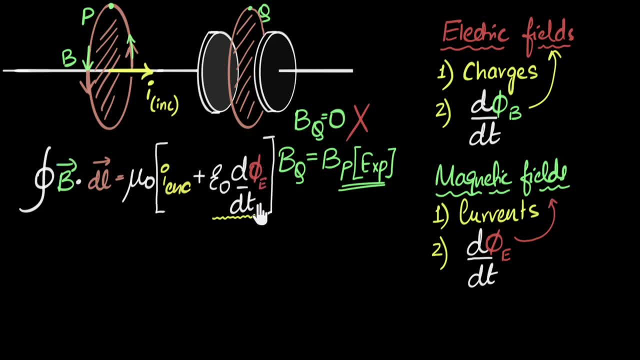 current And therefore this should also have the units of ampere, And you can go ahead and check that. It indeed does have the unit of ampere And it's for this reason Maxwell gave this term a name. He thought this is some kind of current flowing between the capacitor plates and he called it. 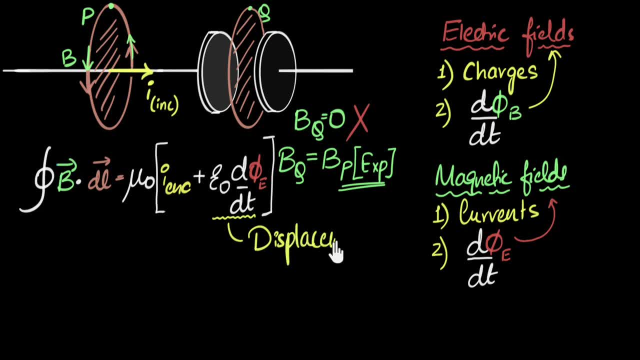 the displacement current, Displacement current, And I always wondered why did he call it that? I read up some articles. I'm not sure how credible this is, but some articles said that back then Maxwell believed that there is ether medium everywhere in the universe, even in between. 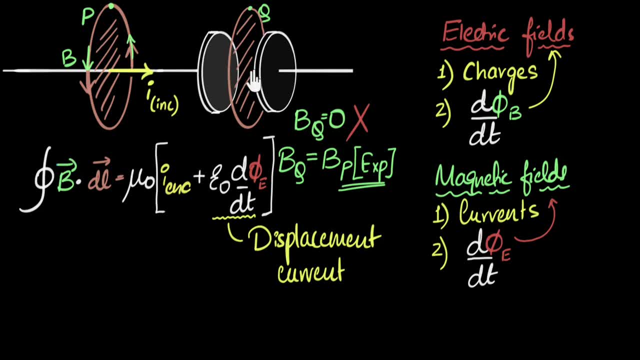 the capacitor And he thought that, as the electric flux is changing, it's the particles of ether that is getting displaced, And maybe that's the reason he thought that there's some kind of current and so he called it the displacement current. But of course today we know there is no ether medium. 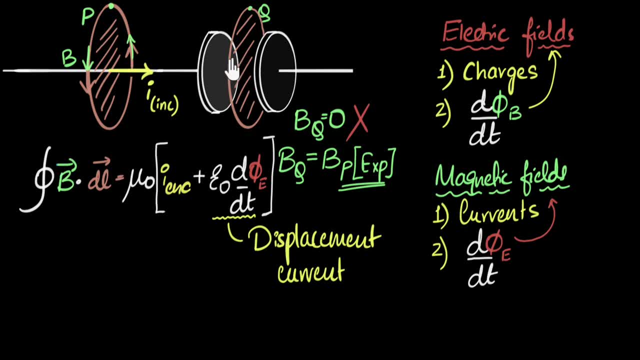 there's truly vacuum in between these two plates and so there is no current. So this is not really any current, but the name is stuck To differentiate this term from the actual current. we also call this the real current or the actual current, conduction current. So conduction current is, you know, the actual. 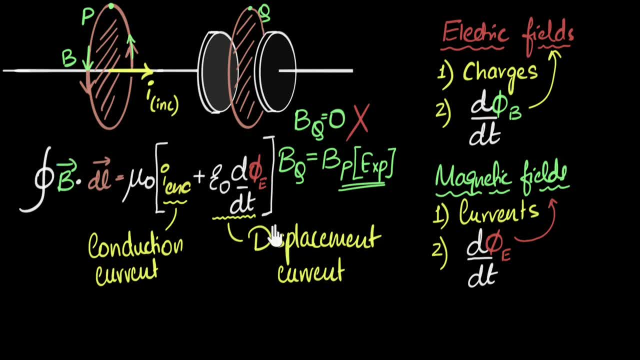 current, the good old, familiar current And displacement. current is just the term that takes care of the changing electric flux that produces magnetic fields. And now, if we go ahead and use this Ampere-Maxwell's law and apply it at point P and point Q, we will indeed see the magnetic fields will be exactly the same. 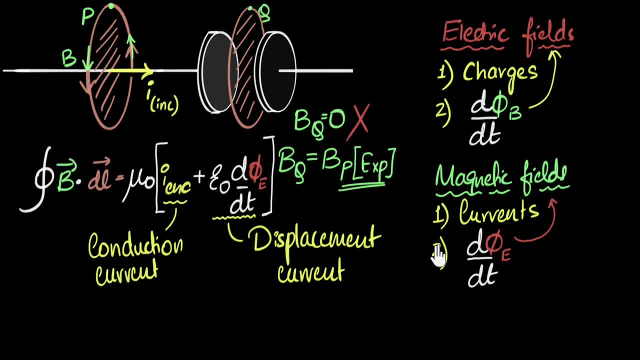 And we'll do that calculation in another video. But long story short, what did we learn? We learned that back then, Ampere and many other people thought that there's only one source of magnetic field- electric current- But today we know that's not true. there's another way to generate magnetic.